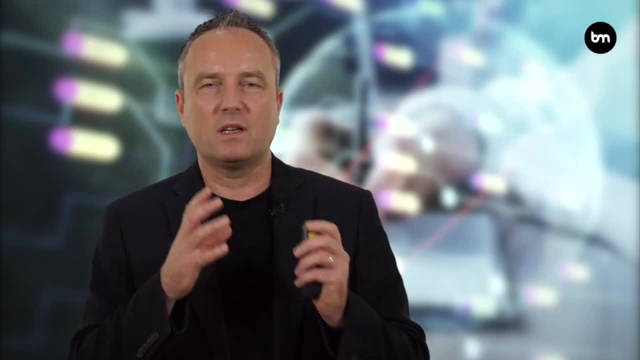 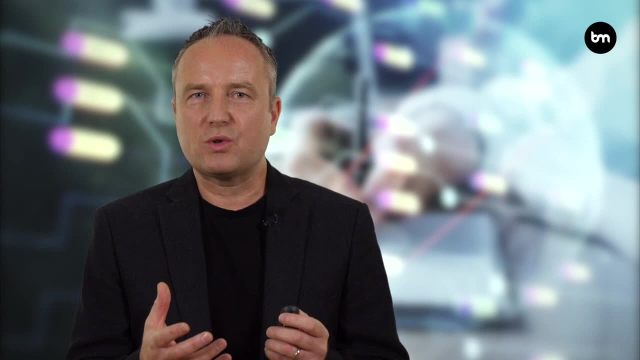 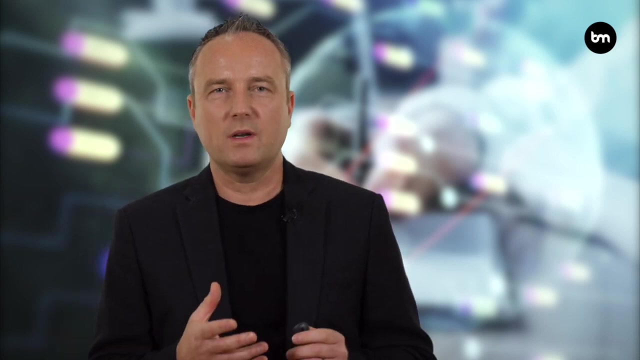 What are the biggest ethical challenges when it comes to artificial intelligence? So in this video, I want to explore some of the biggest challenges in terms of ethics that I see when it comes to AI. The first one is biases, So we need data to train our artificial intelligence. 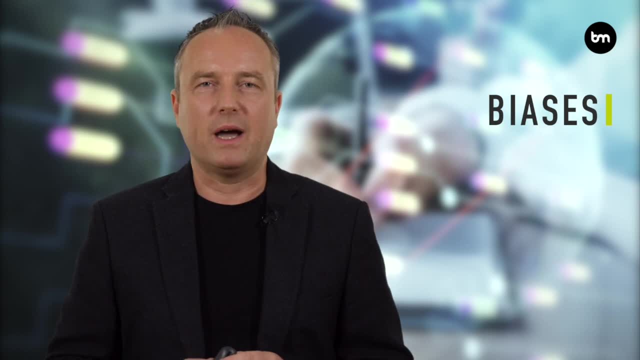 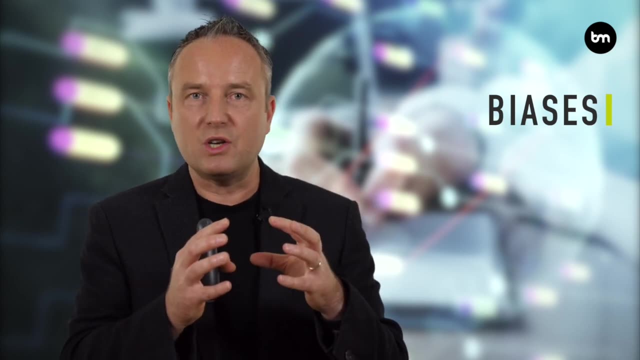 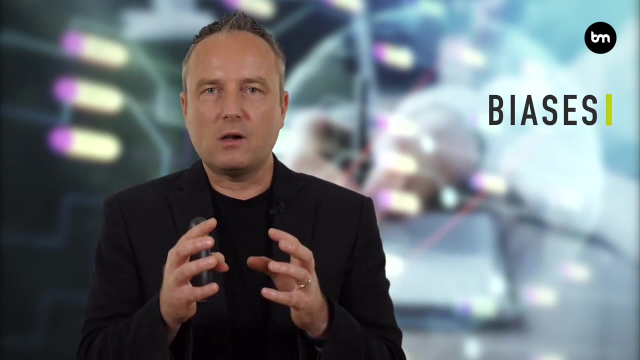 algorithms, and we need to make sure that this data is not biased. We've had this for many years, now that one of the database that uses face images, for example, is called ImageNet, and this had far more white faces than non-white faces. So when we then trained our algorithms to recognize facial 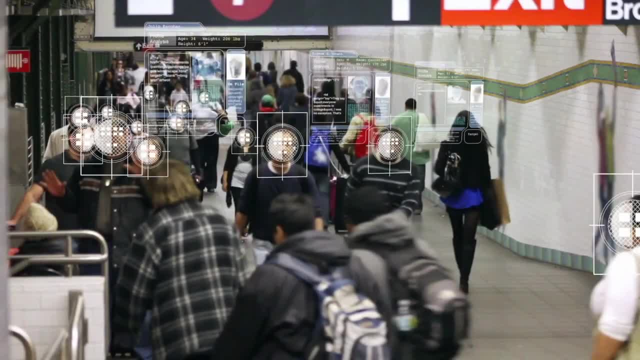 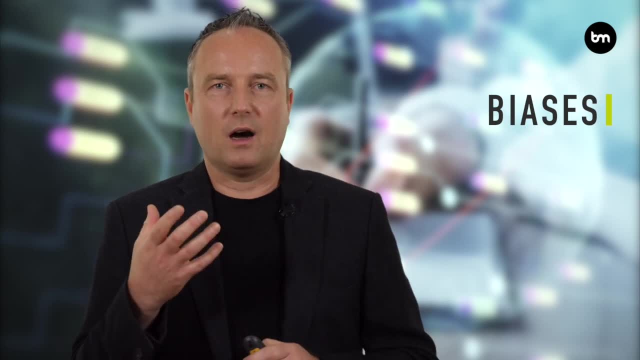 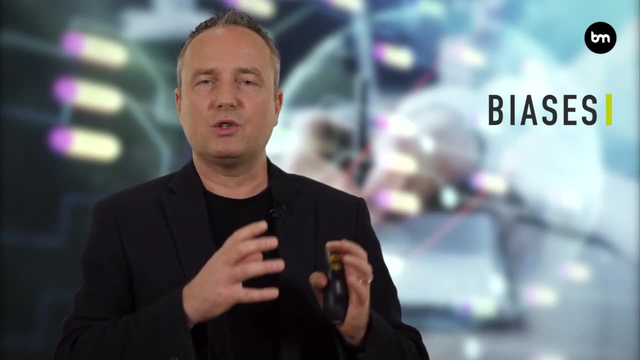 features. for example, those algorithms were not working as well on non-white faces. Then, of course, we can generate algorithms that are in itself biased. So Amazon, for example, has had this: that they're a recruitment was biased towards men, for example, over women, or algorithms like Google search. If 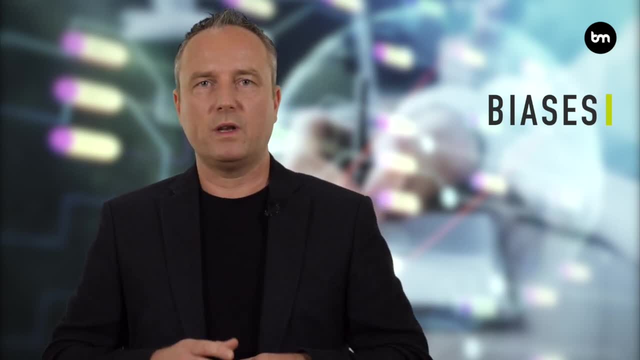 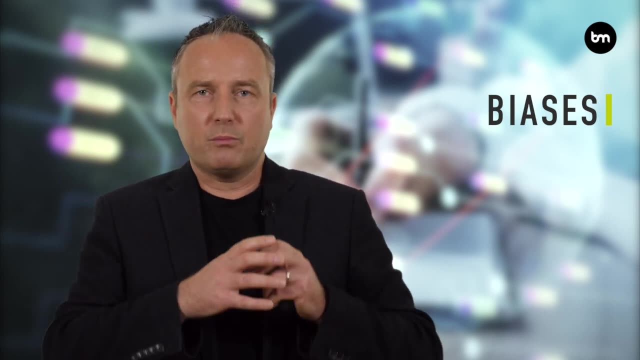 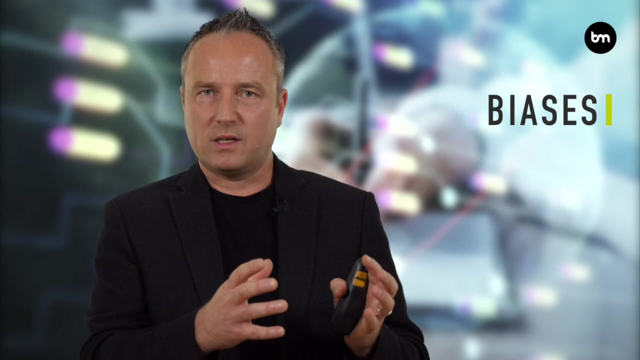 you search for school girls, you get very different images to when you search for school boys, for example, And these are biases that permeate through society and reflect the world we live in. So the challenge is: do we accept this and say these AIs are just trained on the real world? 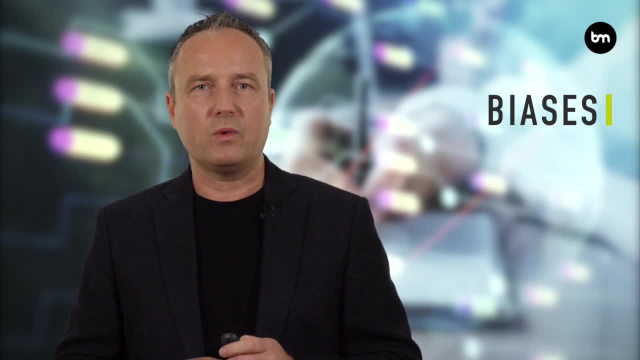 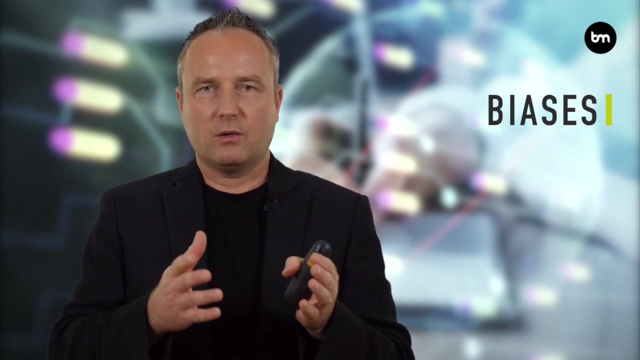 or do we change them? And for me it's really important that we change them and we build AIs that eliminate some of the biases we have. And one of the examples often used this trolley problem, where basically you have the choice, So a trolley is running down a track and you don't have to make a decision, you lead the trolley. 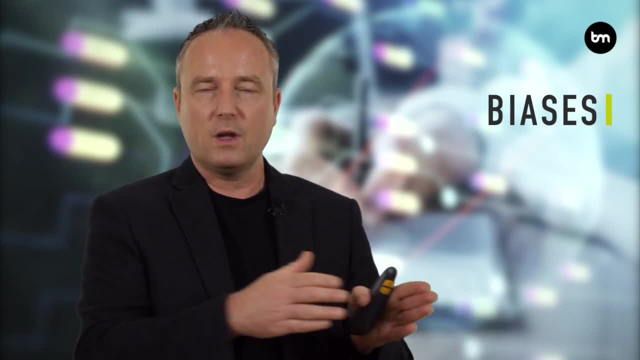 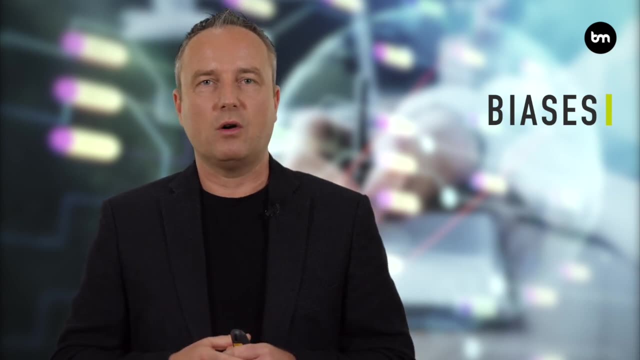 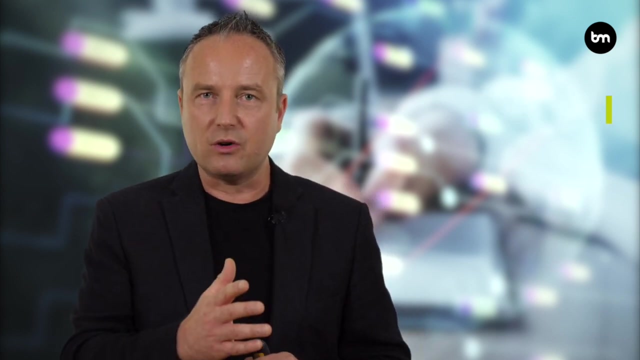 in one way, and it would kill someone you know. or you could send the trolley the other way, and it would kill someone. it would kill five people. but those that you don't know- and this is AIs- in the future will make more decisions, not necessarily as harsh as those, which brings me to the next. 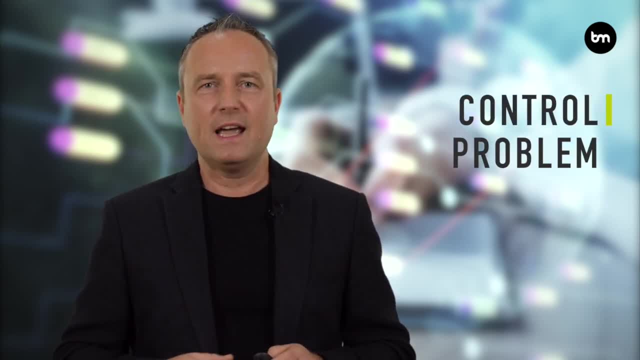 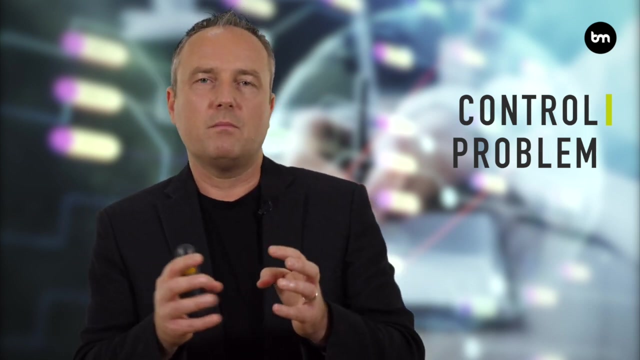 problem, which is this control problem, that it is this whole idea that we leave machines to make increasingly important decision. we talk about moral agency or who is responsible for making those decisions, and at the moment we very often say, okay, we create nice algorithms, but then we let humans make. 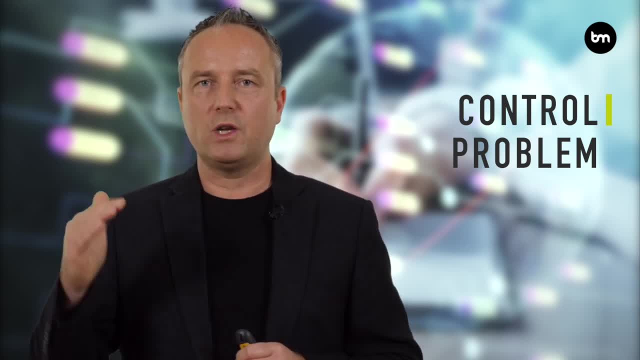 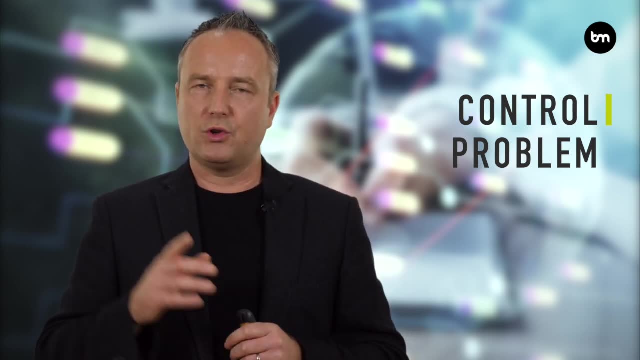 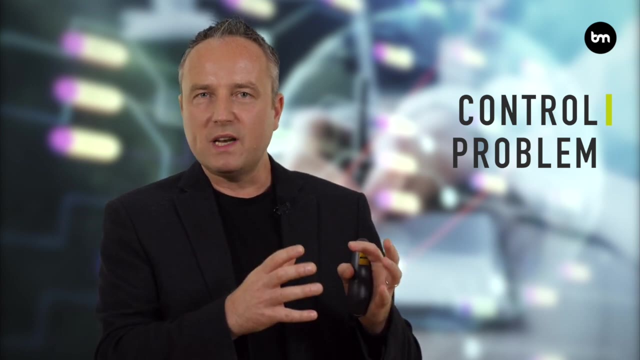 the ultimate choice, very similar to this trolley problem- is if we use autonomous weapons, for example. at the moment there's an international convention that says if you want to use an autonomous drone, for example, that could potentially fire a rocket and kill someone, there needs to be a human in the loop. so the 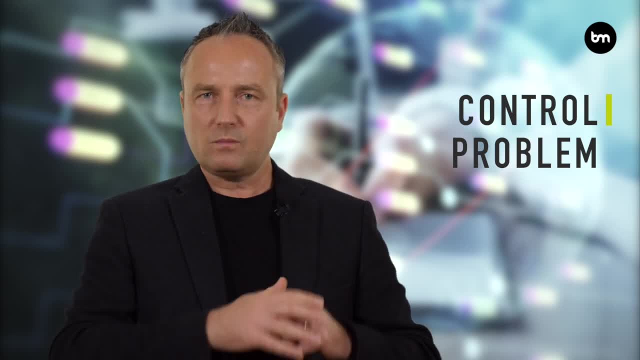 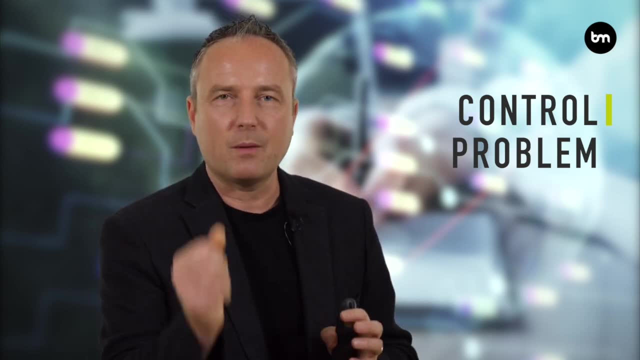 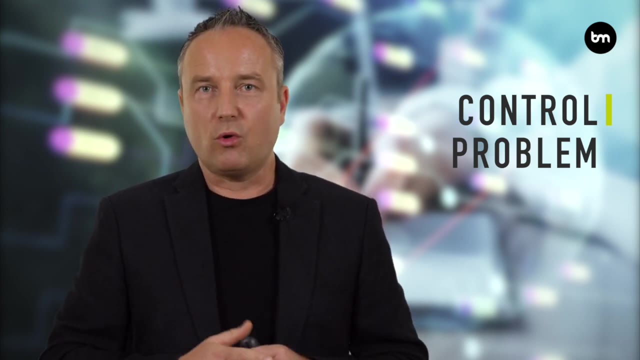 human will make the decision to press the button, and this is how we get around this control problem. the problem today is that AIs now make decisions that have to happen so quickly. so, for example, high-frequency trading- over 90% of all financial trades- are now driven by algorithms, and these make decisions in a split second, so that 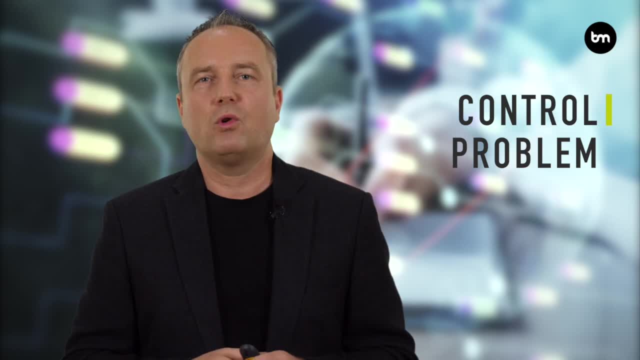 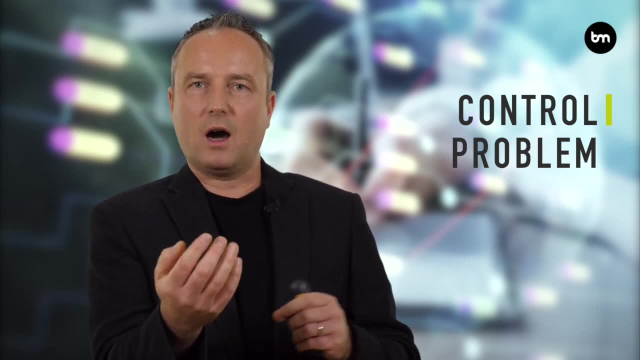 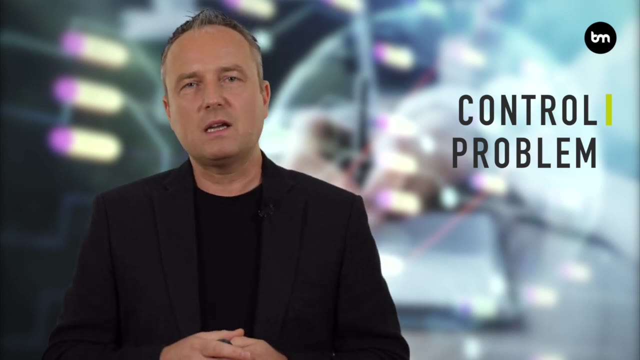 we can't actually have a human in the loop. the same for autonomously driving cars. they have to respond so quickly. if a child runs out in front of the car, the car needs to react immediately and we can't say, okay, you now make have to make a decision. so this makes it an interesting ethical challenge: how much. 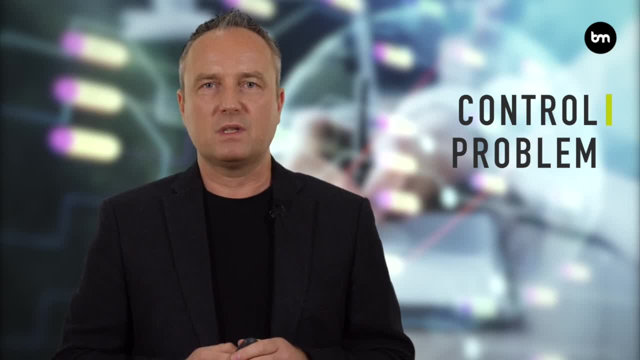 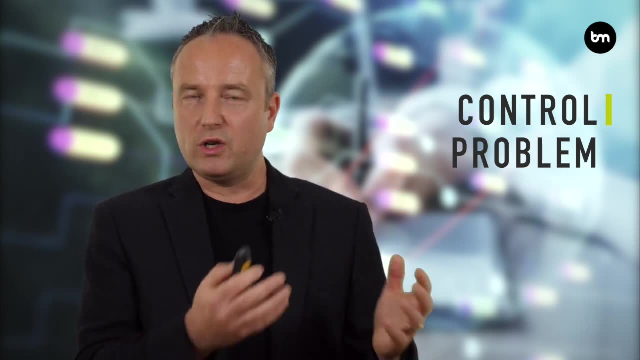 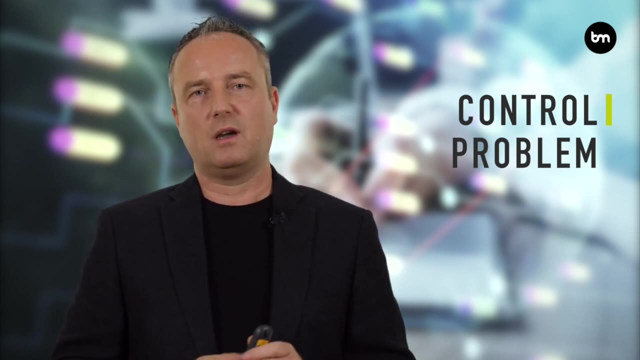 of this do we then program into the algorithms? do we protect the driver? do we protect the pedestrian? and these are challenges that are quite unique to AIs, because when we, when we humans- make them, we make them in a split second and we don't have to prejudge some of these decisions that we'll make in the future. 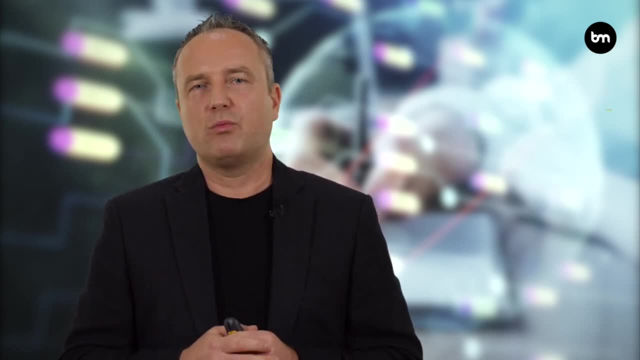 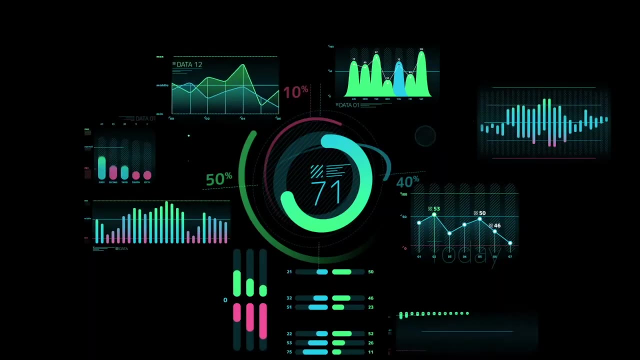 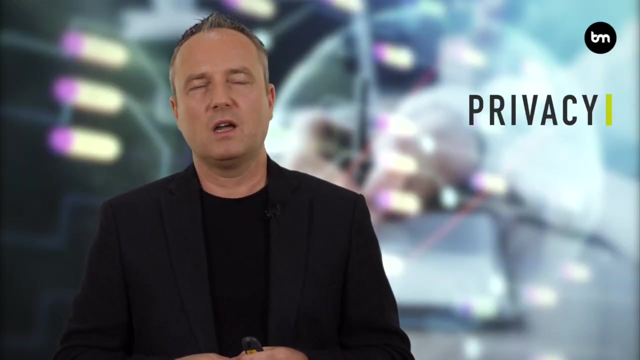 another ethical challenge is around privacy and especially the consent. so when we use data that we use to train the AIs, where's this data come from? and then how do we use this data? and sometimes we make this assumption that we have humans with full mental capabilities that can make those choices. 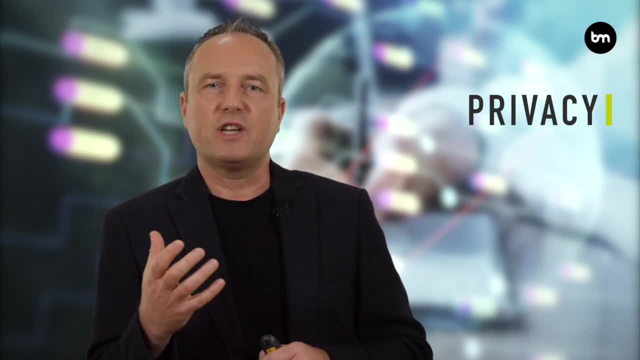 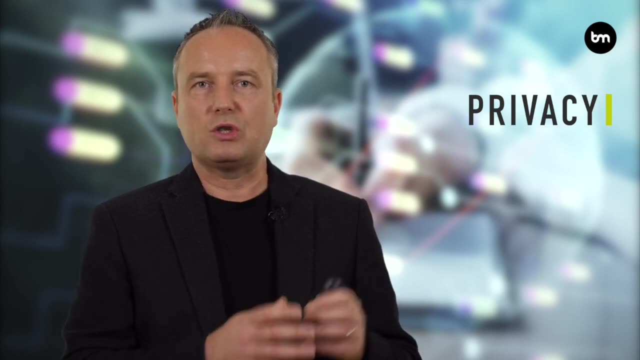 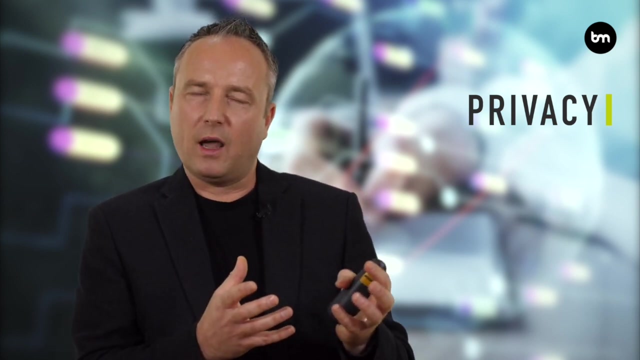 that can say: I want to use this AI. the challenge is when we don't have this. so, for example, Barbie and now has an AI enabled toy, a door that children can speak to. what's this now mean in terms of ethics? because suddenly you have an algorithm that is collecting data. maybe your child is. 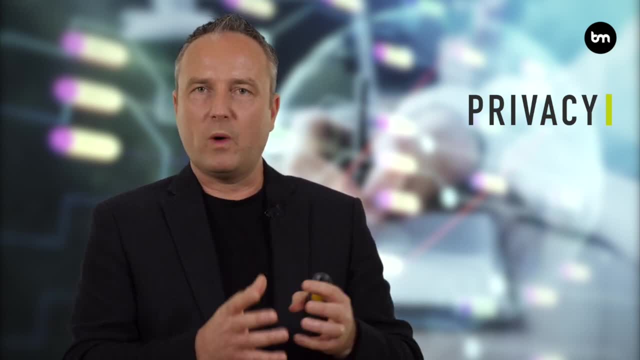 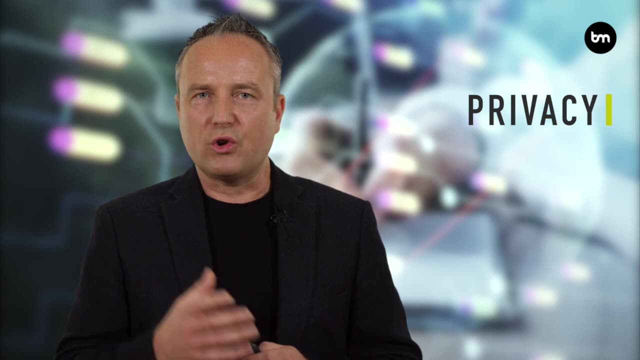 having some intimate conversations with this toy. where's this data going? how's this being used? how is this influencing the child, which I think is really important to to consider? the other thing is: how do we use some of the data we now have and some of the capabilities, things like face recognition, for example, or there are. 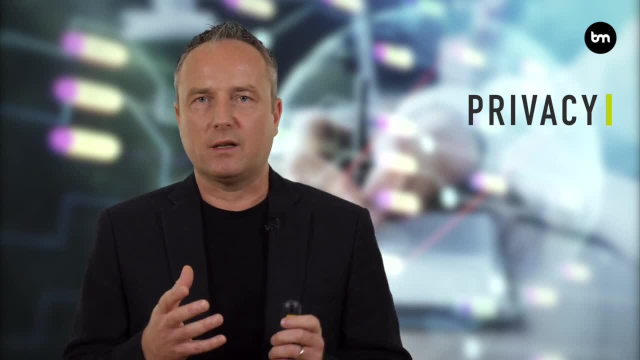 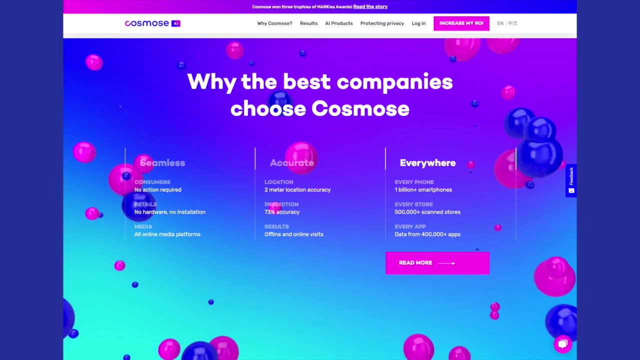 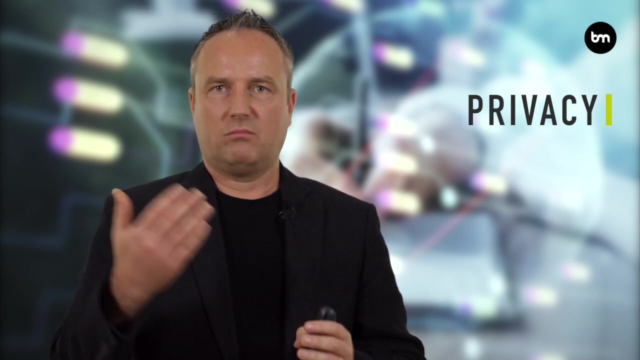 many companies and aggregate data that, again, many people are not even aware of. there's a company called cosmos AI that is collecting data from thousands of the free apps that we download onto our phones and we think, hey, what's the harm in those? I just use this app and then I'm just, you know, I'm just using this app and 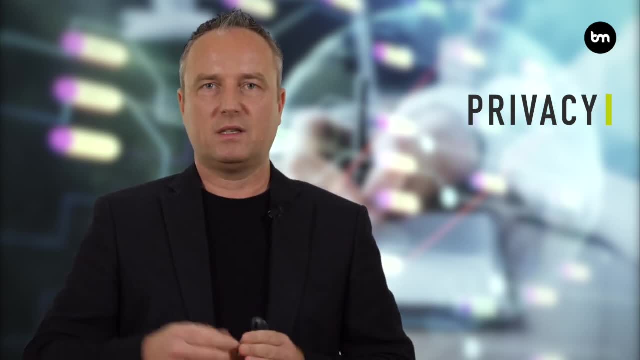 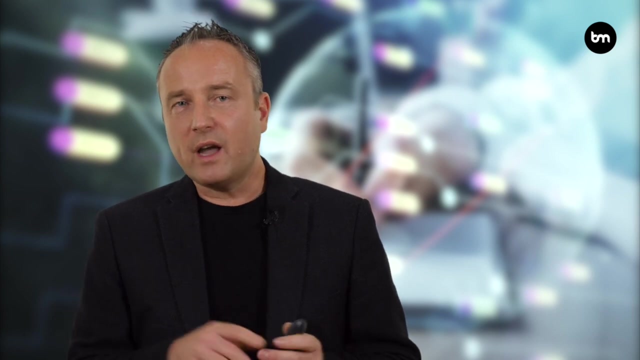 but all of these apps are now collecting data and they're selling this data to cosmos AI, which is an aggregating all of this data to get a very detailed understanding of customers and is selling this. so for me, we need to think about transparency and privacy in this context of AI, another ethical challenge. 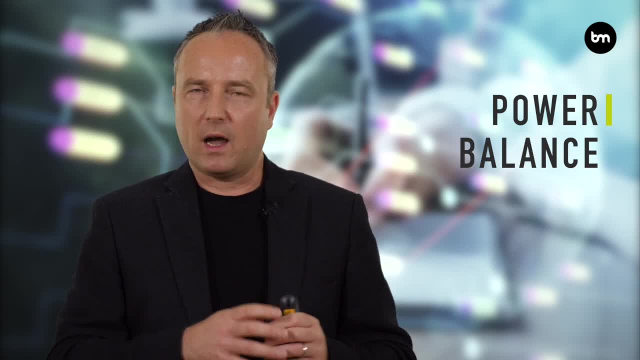 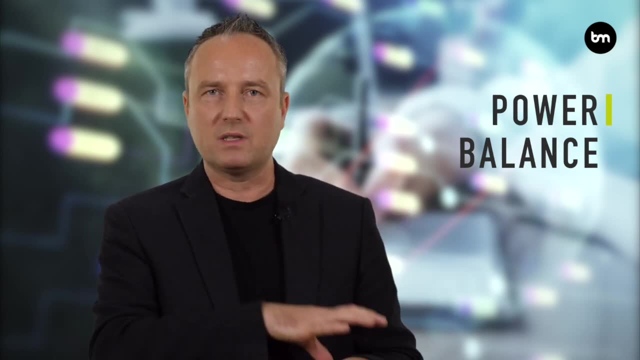 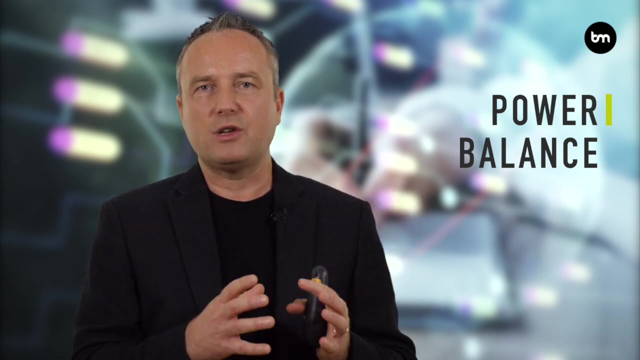 is the, the power balance. we now have companies that are building big monopolies and becoming extremely powerful companies like Amazon, Facebook, Google, who are able to use those AIs, and they are out competing most other companies. we also have countries. China, for example, has a hugely ambitious AI strategy that is supported by government and President Putin for 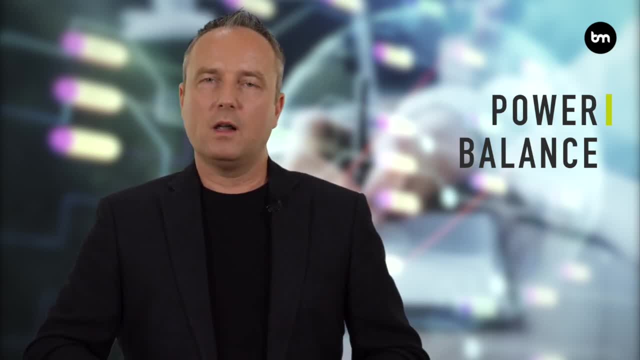 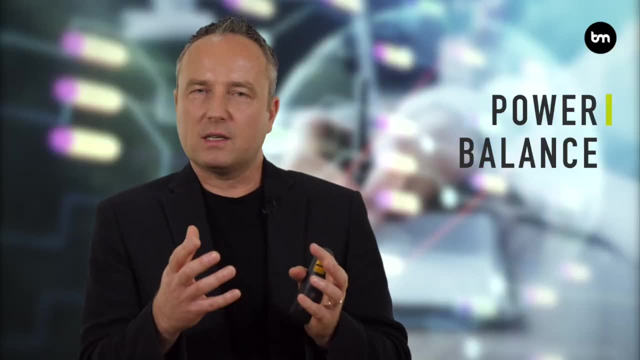 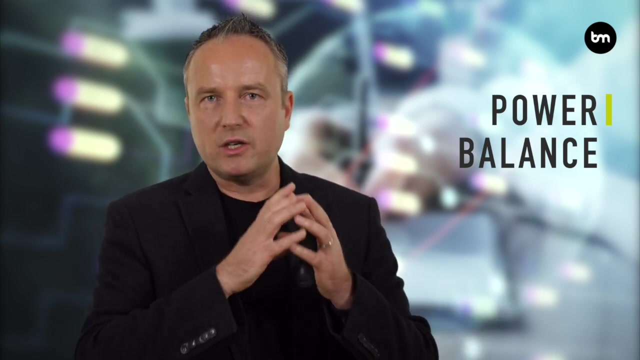 example of Russia, said that whoever will win the race in AI will probably become the ruler of the world. so there's this challenge: how do we make sure that some of the monopolies we're generating, that they are actually distributing the wealth more equally and that we are not having a few countries around the 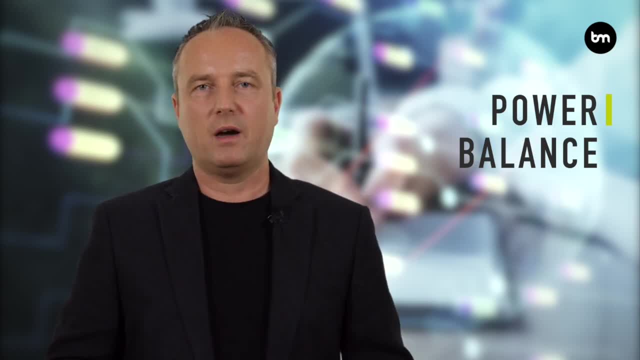 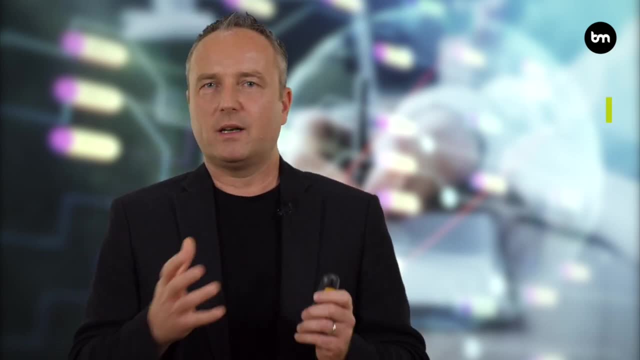 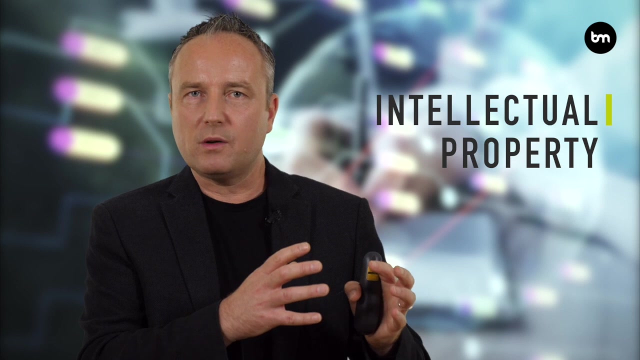 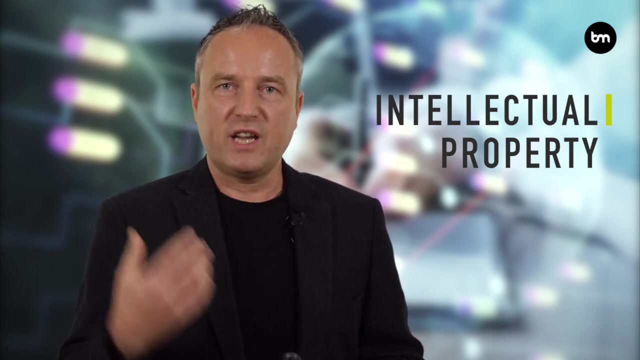 world racing ahead whereas other countries are being left behind. so this is another challenge. another thing to worry about is ownership and intellect, intellectual property, for example. so, and which comes back to again, who is responsible for some of the things that AIs are creating? so we can now use artificial intelligence to create text. 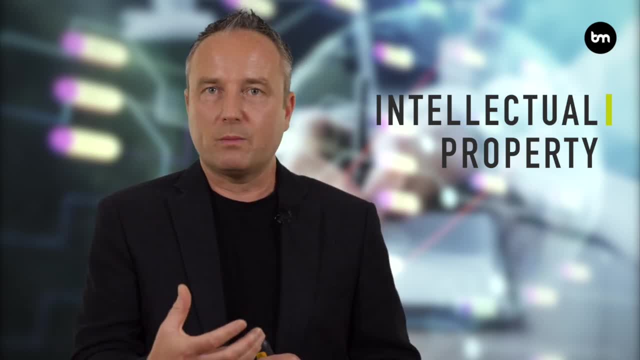 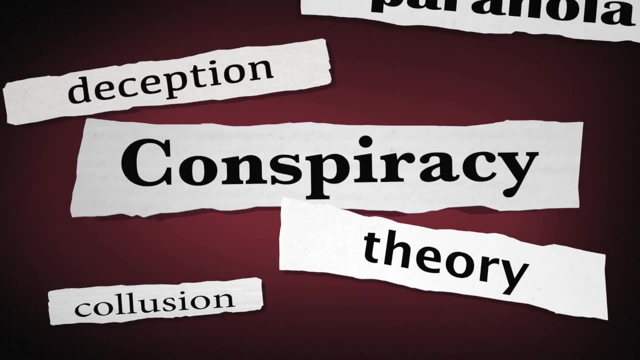 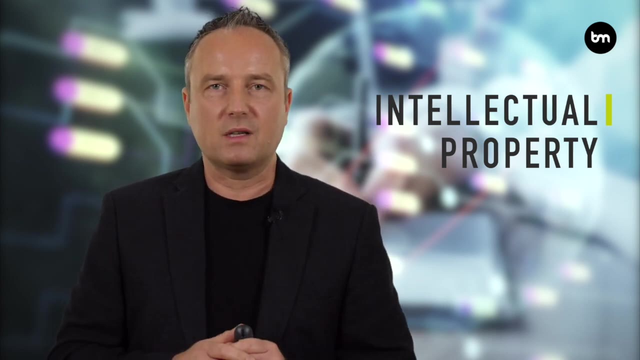 automatically, which means we can have automatic Twitter bots that might spread fake news. we now have deepfakes that even use AI to create deepfake videos of people doing some is talking about things on YouTube that is not. they're not real. we now have AIs that can create art and 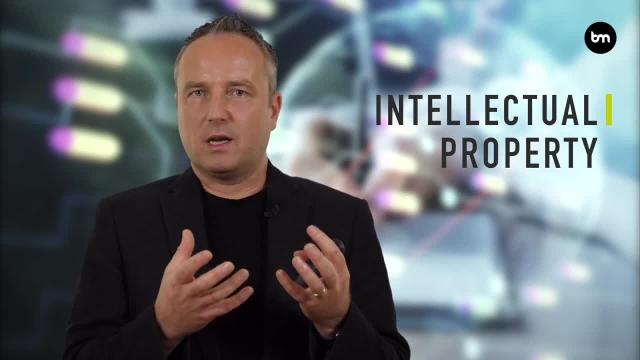 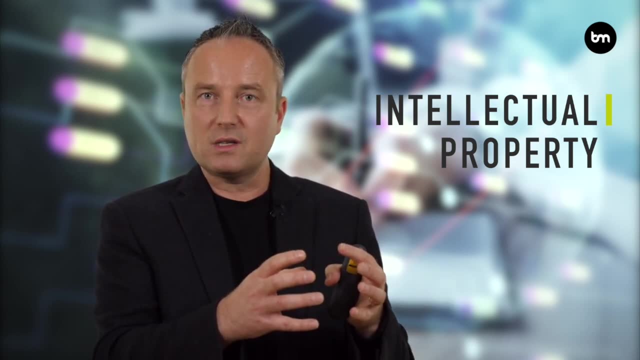 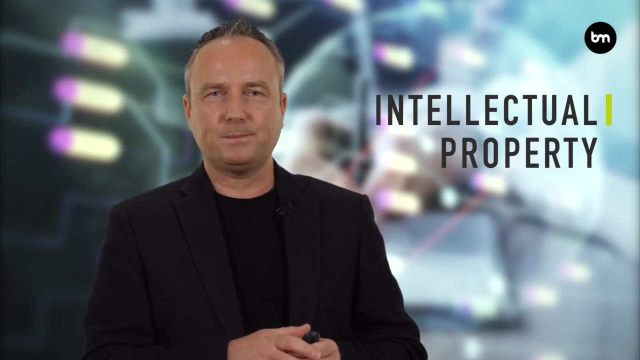 music and for me there are a few challenges here. when I have an AI that writes a new piece of music, who actually owns this, who has the intellectual property right for this and therefore potentially gets paid for it? but also who is responsible for this? so if I am creating, if I have a news bot for 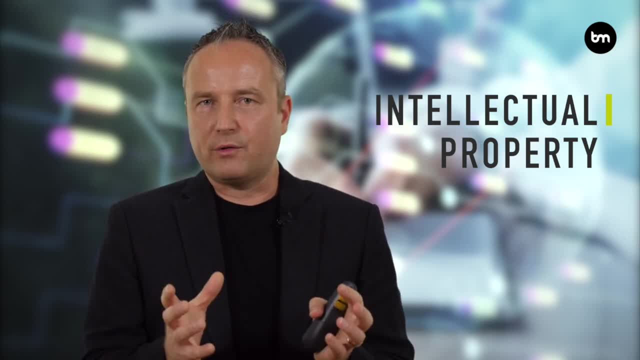 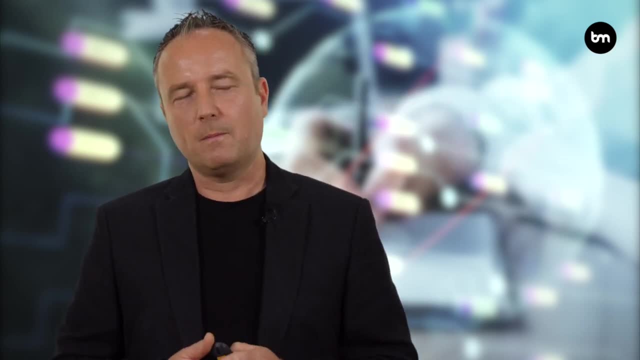 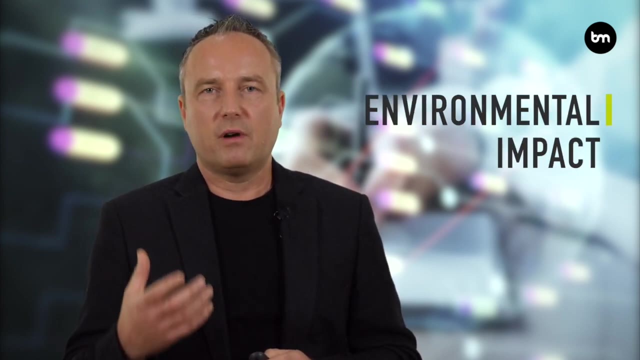 example, that writes news articles automatically, and these are fake news that are then spreading across the internet. who is ultimately responsible for this? so this is a big challenge for me. my other challenge when it comes to ethics around AI is the environmental impact. we sometimes think that we are using data somewhere on a cloud computer. 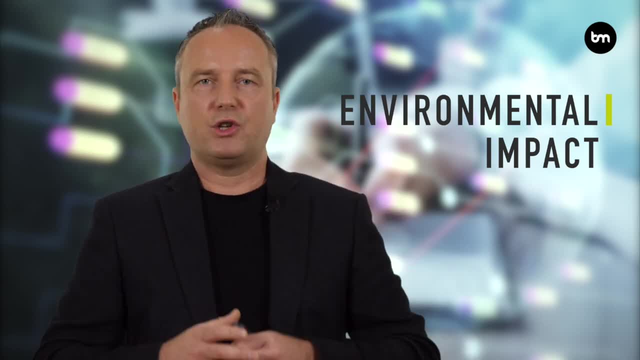 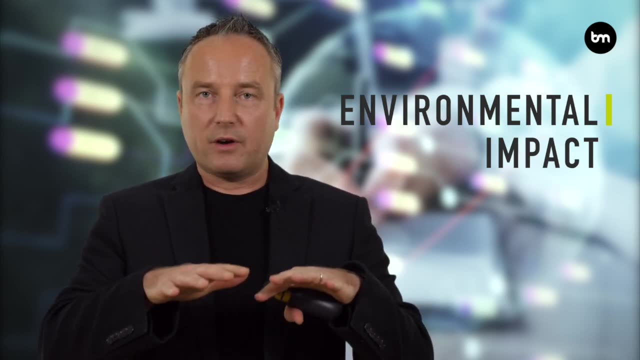 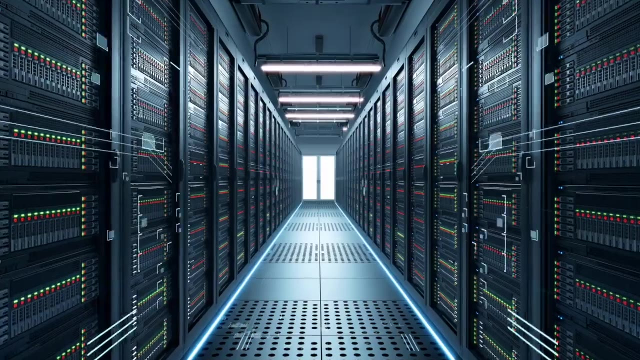 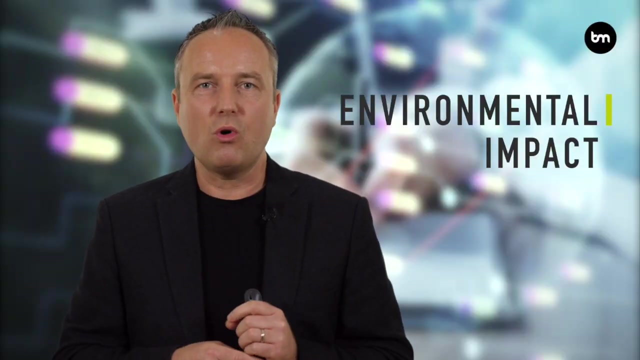 to train an algorithm that then is used to run recommendation engines on our website, and sometimes we don't even think that there's an in environmental cost to all of this, but those computer centers that run our cloud infrastructure are very power hungry, and training in AI, for example, can create 17 times more carbon emission. 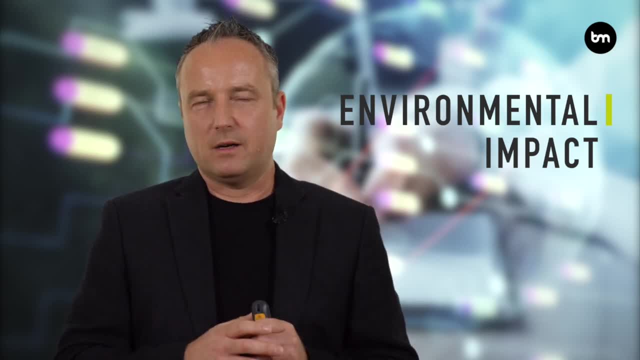 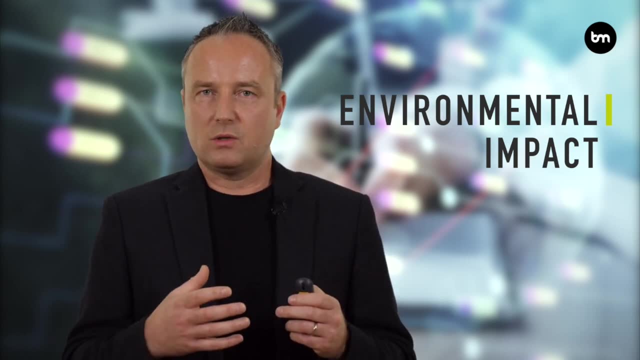 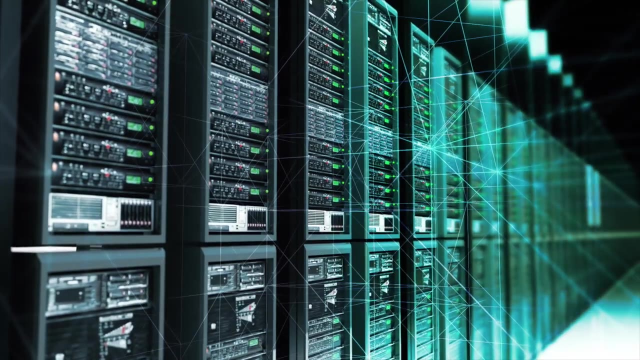 than the average American does in about a year. So this is something we need to consider: that there's an environmental cost and for me, what we need to do is to really think about: is this the right use of this energy? Can we use the energy to actually solve some of the biggest problems we have in the